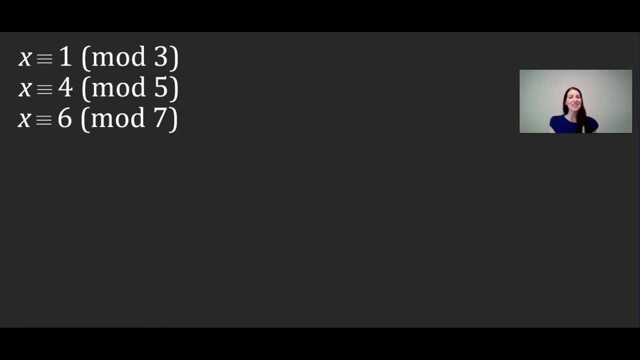 Hi everyone, it's Calculus by Christy, But actually in this video we're going to take a little break from calculus and do some modular arithmetic. And you may be thinking: why is she doing this? Why is she taking a break from calculus? Well, not only am I a calculus teacher, but I'm actually also a high school math team coach, And modular arithmetic is something that shows up, And specifically what's called the Chinese remainder theorem shows up. But I would like to 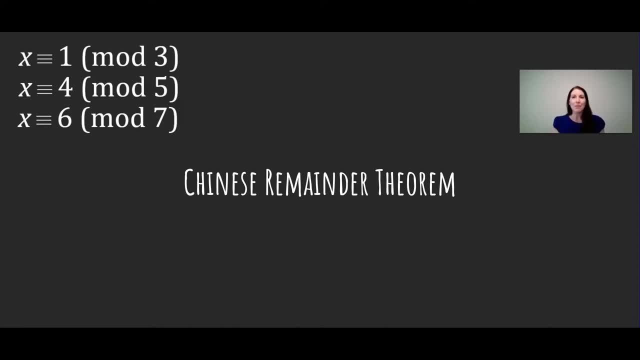 take a moment to give credit where credit is due, Because the Chinese remainder theorem- even though that is the name it- was a theorem by Sun Tzu And I would like to give some credit because it seems like his name has been wiped away from this theorem. So, instead of calling it the Chinese remainder theorem, because I want to give credit where credit is due, I would like to call it the Sun Tzu theorem. So, in order to get started to solve this. well, it is a 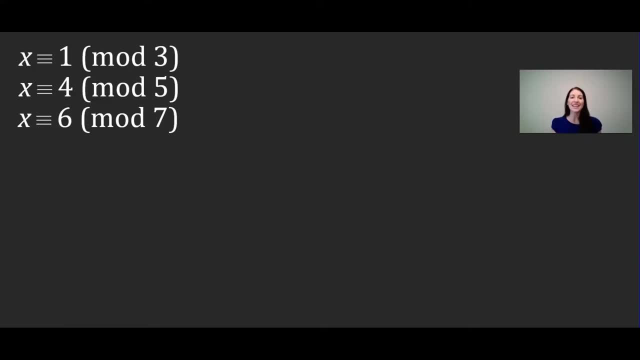 multiple linear congruence problem And it kind of can be tricky, But I hope that by explaining it I can explain it in a really, really simplified way that is easy to understand. That is my hope. If that is what happens, please leave a comment down below and let me know if this was easy to understand and that helped you out. So before we get to this problem, I would like to talk about any general problem here. So let's say I 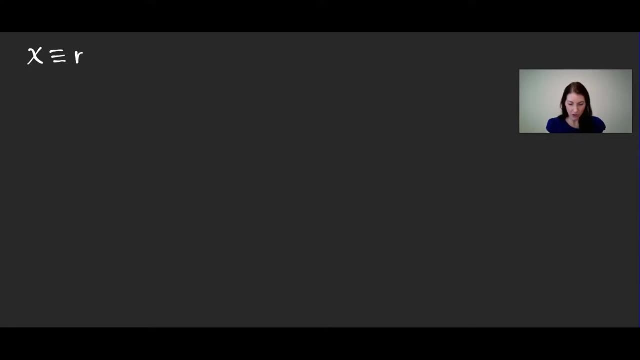 had x is congruent to r1 mod m1, where r is the remainder. So we've got a second remainder in a different mod And then we've got a third remainder in a third mod. So in order to be able to use this Sun Tzu theorem, we first need to make sure that the 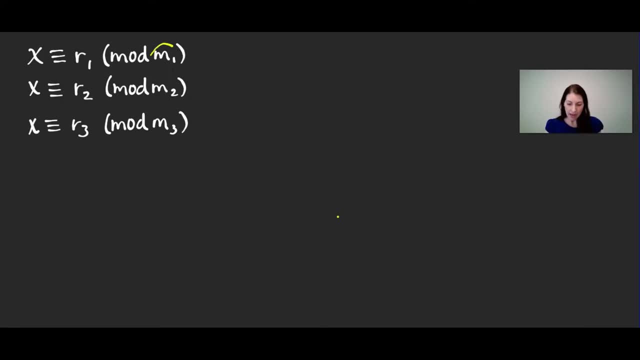 are relatively prime. That means, whenever I pair up these mods, the greatest common divisor between m1 and m2, it needs to be one and the same with m2 and m3, and then the same with m1 and m3. So the greatest common divisor should only be one, And if that is true, then we can use this theorem. So we always want to, you know, make sure that we have that first. All right, so next up we're going to look at the 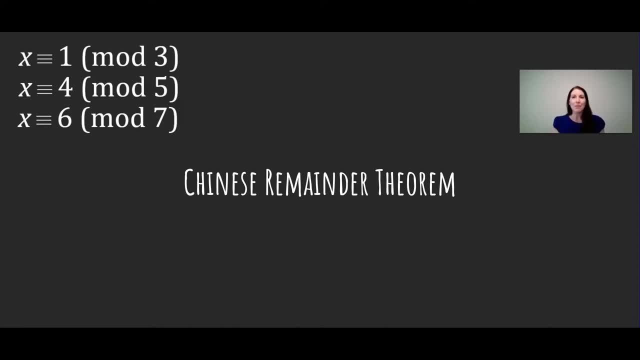 take a moment to give credit where credit is due, Because the Chinese remainder theorem- even though that is the name it- was a theorem by Sun Tzu And I would like to give some credit because it seems like his name has been wiped away from this theorem. So, instead of calling it the Chinese remainder theorem, because I want to give credit where credit is due, I would like to call it the Sun Tzu theorem. So, in order to get started to solve this. well, it is a 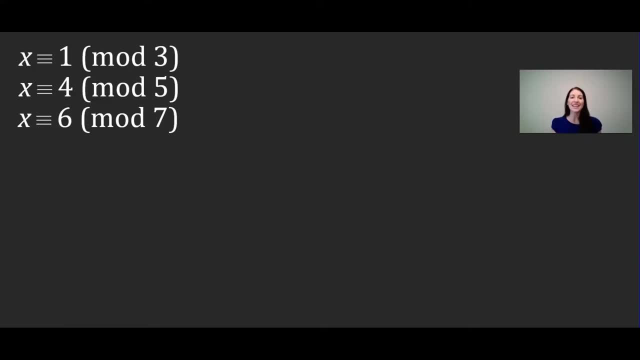 multiple linear congruence problem And it kind of can be tricky, But I hope that by explaining it I can explain it in a really, really simplified way that is easy to understand. That is my hope. If that is what happens, please leave a comment down below and let me know if this was easy to understand and that helped you out. So before we get to this problem, I would like to talk about any general problem here. So let's say I 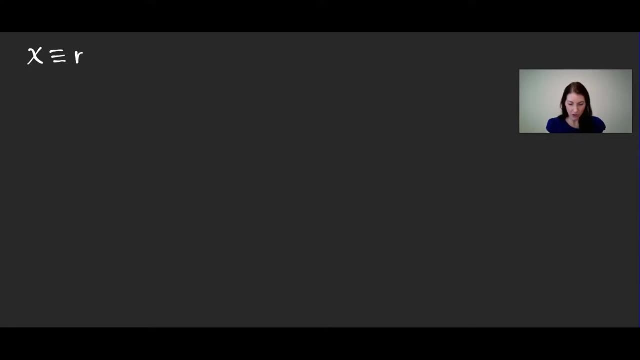 had x is congruent to r1 mod m1, where r is the remainder. So we've got a second remainder in a different mod And then we've got a third remainder in a third mod. So in order to be able to use this Sun Tzu theorem, we first need to make sure that the 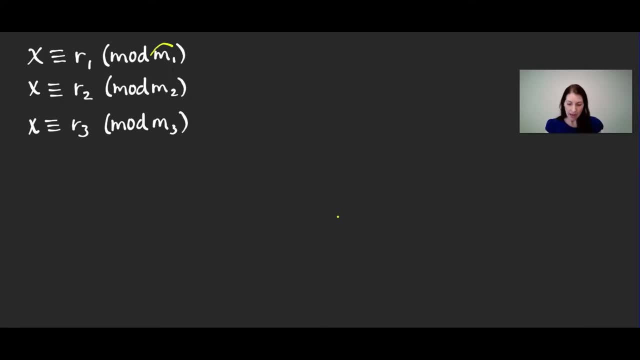 synonyms of the two modes are relatively prime. That means whenever I pair up these mods, the greatest common divisor between m1 and m2 needs to be one and the same with m2 and m3, and then the same with m1 and m3. So the greatest common divisor should only be one, And if that is true, then we can use this. 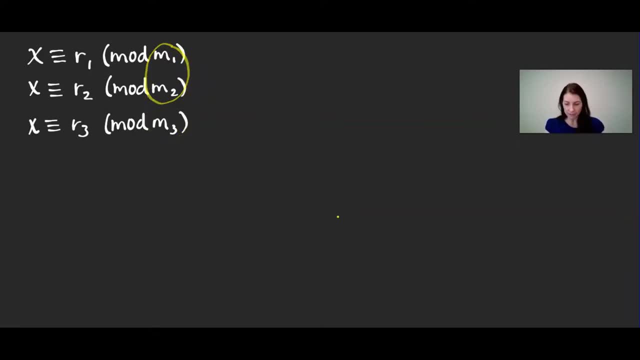 theorem. So we always want to, you know, make sure that we have that first. All right, so next up, what I do is I create a table, and creating this table just kind of helps me organize all the information that I will use. So the first column is where I put all the remainders, So I'll put the 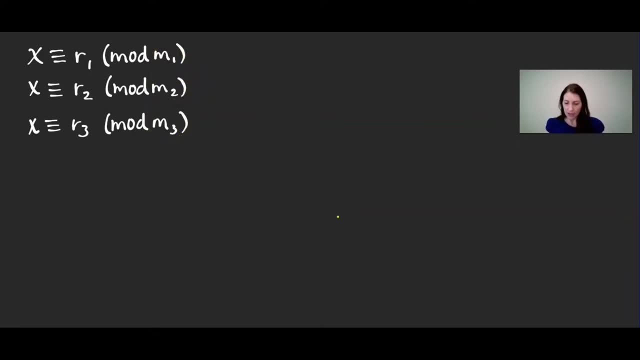 to you know, make sure that we have that first. All right, so next up, what I do is I create a table, and creating this table just kind of helps me organize all the information that I will use. So the first column is where I put all the remainders. So I'll put the RIs. So first I will. 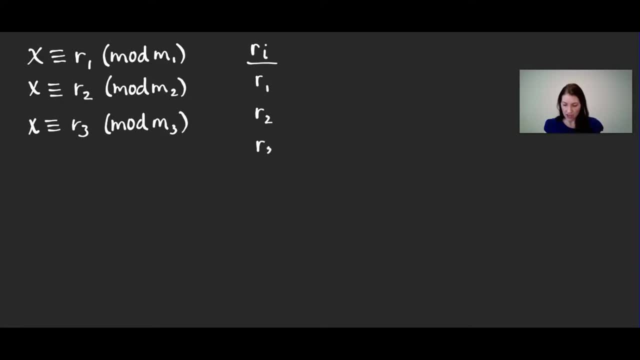 have R1, and then R2, and then R3, which are my remainders over here in my original problem. Next up I will put MI and let me explain what that is. So first we have this unique modulo for each problem and I'm going to call that M. To get M, I would take the product of M1 times M2. 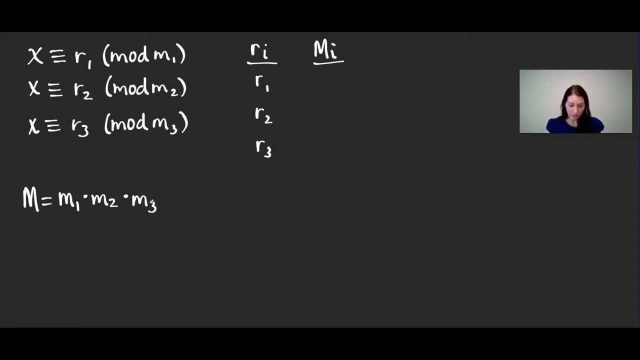 times M3.. Then to find MI, what I'm going to do is I'm going to take that unique modulo M and divide by the product of M1 times M2 times M3.. So I'm going to take that unique modulo M. 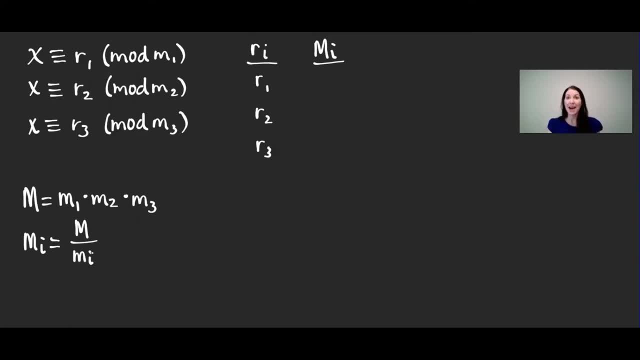 and divide by the product of M1 times M2 times M3.. So I'm going to take that unique modulo M and divide by whatever MI is. So for example, to get M1, I would take M and divide it by the mod on the very first linear congruence. Now, if you think about that, if that is M1 times M2, 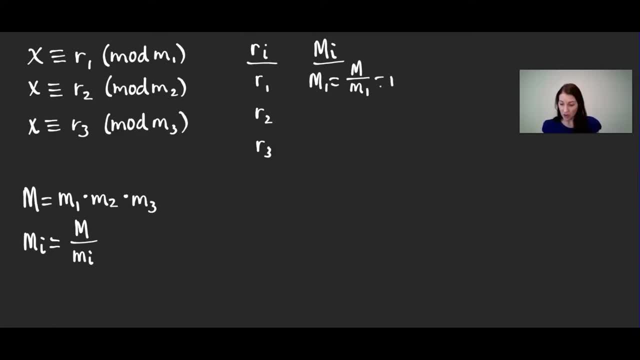 times M3, divided by M1, that leaves you with M2 times M3. Keep this in mind when we go to do the actual problem. So then, therefore, M2 in a similar way would be M1 times M3, and then M3 is going to be. 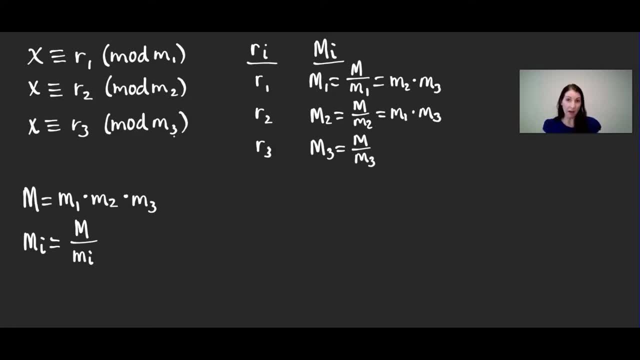 our unique modulo, divided by the mod on the third congruence, which would be M1 times M2.. All right, so that's going to be my second column as I organize all of this information, and my third column is going to be my second column as I organize all of this information, So I'm going to. 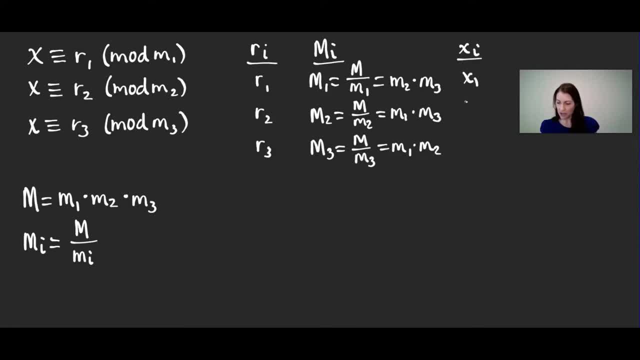 be my second column as I organize all of this information, and my third column is going to be XI, And what these are going to be are these are going to be my inverses of MI, and I'll show you that when we get to the actual problem, Then what we're going to do is we are going to take the 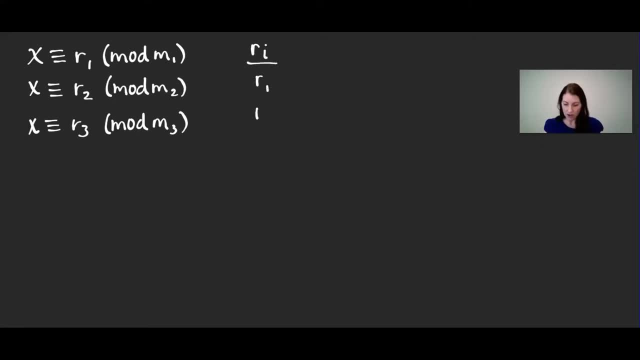 R i's. So first I will have R1, and then R2, and then R3, which are my remainders over here in my original problem. Next up I will put M i and let me explain what that is. So first we have this: 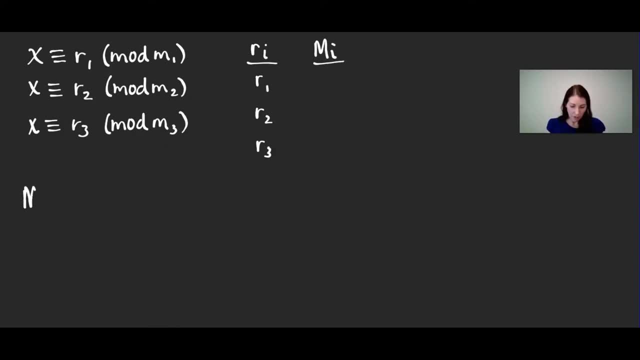 unique modulo for each problem and I'm going to call that M. To get M, I would take the product of M1 times M2, times M3.. Then to find M- i. what I'm going to do is I'm going to take that unique. 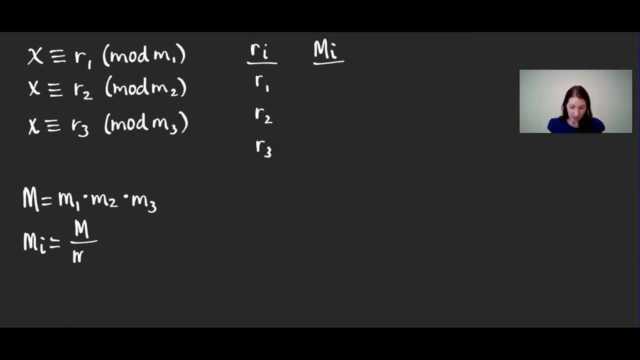 modulo M and divide by whatever M i is. So for example, to get M1, I would take M and divide it by the mod on the very first linear congruence. Now, if you think about that, if that is M1 times M2, 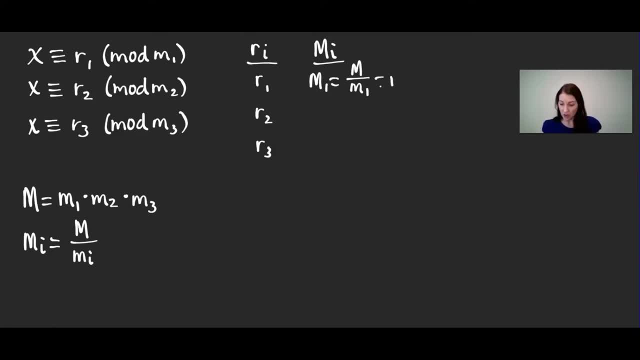 times M3, divided by M1, that leaves you with M2 times M3.. Keep this in mind when we go to the next problem. So I'm going to take the product of M1 times M2 times M3, and divide it. 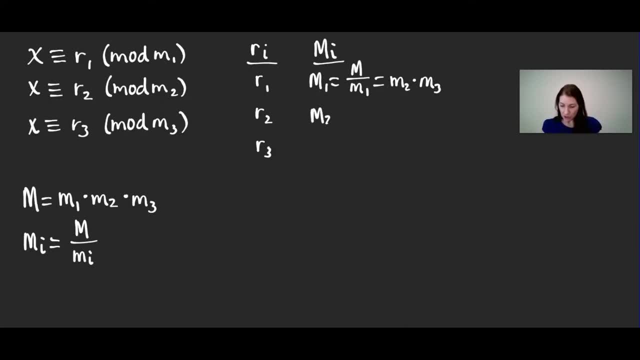 by the mod on the very first linear congruence. Now, if you think about that, if that is M1 times M2 times M3, to do the actual problem, So then therefore M2 in a similar way would be M1 times M3.. 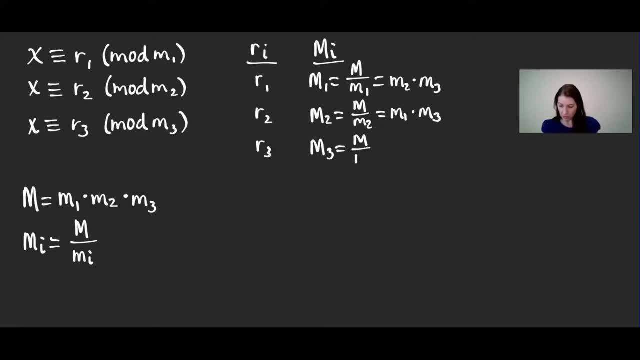 And then M3 is going to be our unique modulo, divided by the mod on the third congruence, which would be M1 times M2.. All right, so that's going to be my second column as I organize all of this information, And my third column is going to be my second column as I organize all of this. 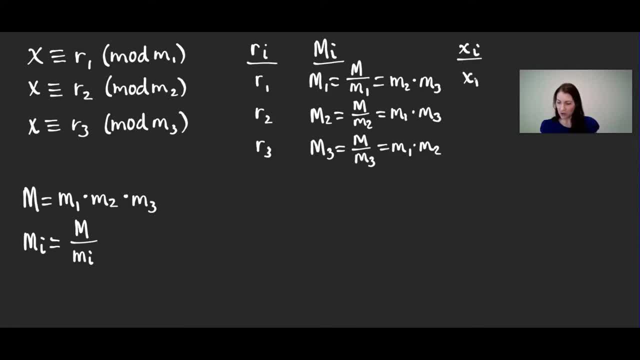 column is going to be xi, and what these are going to be are: these are going to be my inverses of mi, and i'll show you that when we get to the actual problem, then what we're going to do is we are going to take the product of each of these three things. so i'm going to 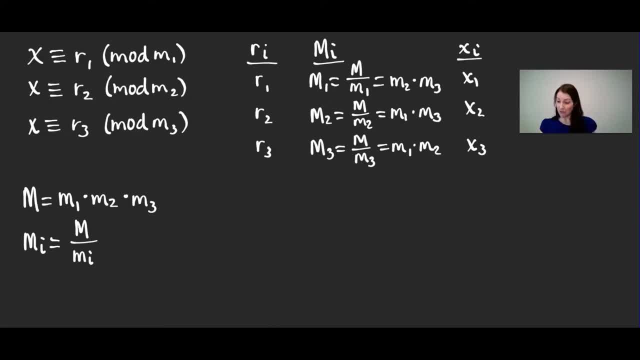 product of each of these three things. So I'm going to move myself real quick down here because I ran out of room And in this last column it's going to be the product of RI times, MI, times XI. So we'll have for our first. 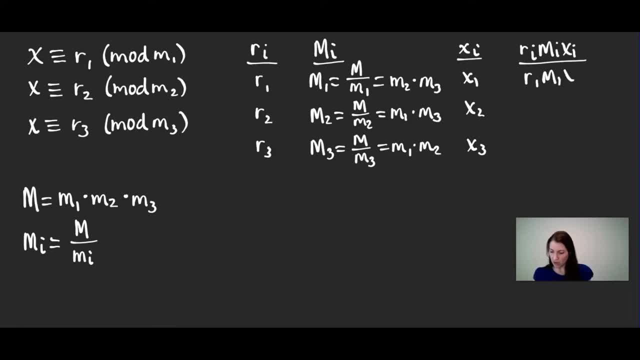 row, then, is R1 times M1 times X1, and so forth down the column here. Finally, what we will do then is we are going to take the sum of all of these three terms. So what that means is we're going to do the summation here. take the sum, where I goes from one to 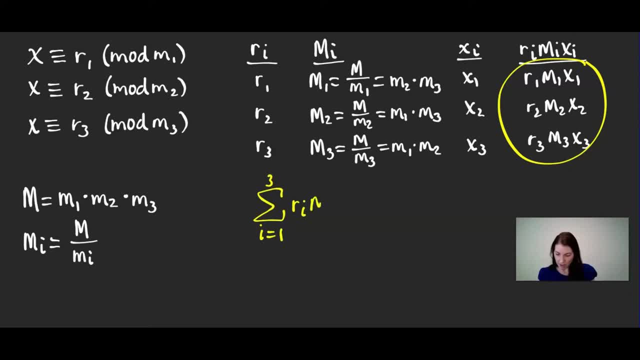 three of RI, MI and XI, and that sum, when taken in the mod of our unique modulus over here, is going to give us what X is equal to, which is what we're trying to solve for. All right, let's take all of. 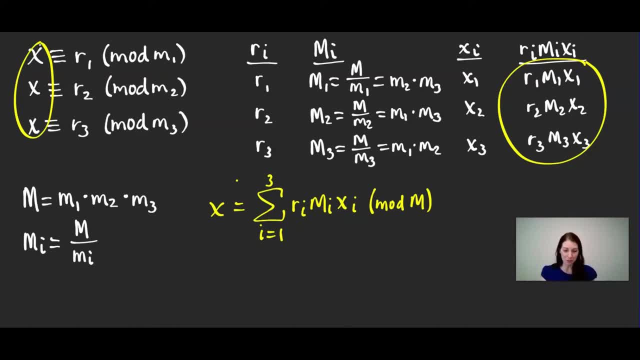 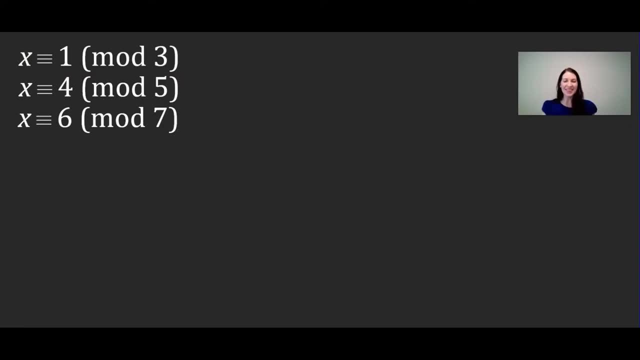 this great information and let's apply it to our original problem. So let's head back and I'll go ahead and move myself back up here and we'll continue on with this problem. So the first thing I write out is: I'm going to write out our remainders, so that's going to be 1 and 4 and 6.. 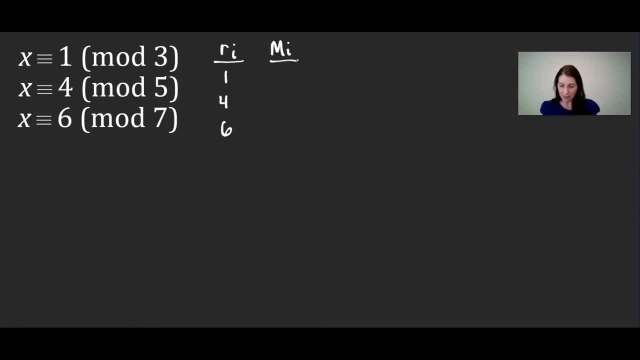 Next are going to be my MIs And even though, as you saw, it's really the product of the other two moduli, I am going to write out what that unit is, And this is U of I除ig of MSI, which is vistilliani. That's something that's going to be inMicom. This is a product of these two moduli and that's what you, inMi, can convert into this second, which, as you can tell O of. so I simply cancel out all of this and 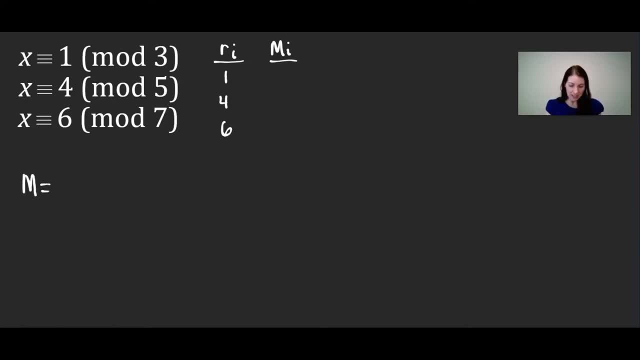 out what that unique modulus m is, because we will need to use it later and that's going to be the product of the three moduli and in our problem here we're going to have 105.. All right, so for our first m1, it's going to be the product of 5 and 7 or 35.. For the next one, it's going to be: 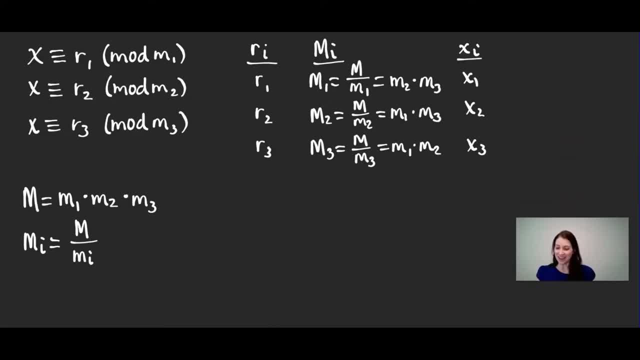 move myself real quick down here, because i ran out of room and in this last column it's going to be the product of ri times mi times xi, so we'll have for our first row. then is r 1 times m, 1 times x, 1, and so forth down the column here. 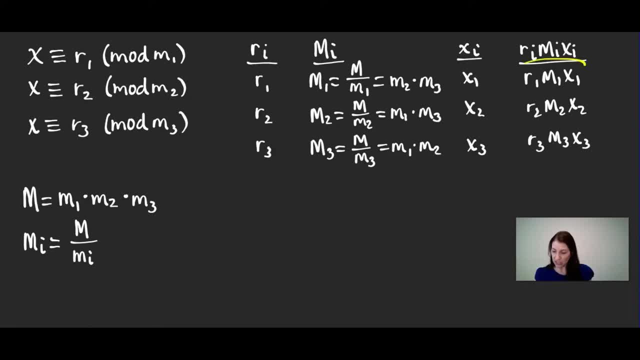 finally, what we will do then is we are going to take the sum of all of these three terms. okay, so these are my installs here, and what i'm going to take are i'm going to take all of the things in here and i'm going to take the sum of my installs, okay, so the next thing that you do then is to stop under my class and then two more from that future variable, and it's gonna be this next columnm that we're going to take. 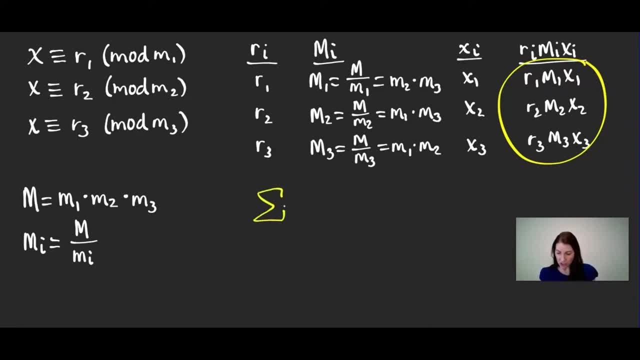 up and look at this again after i input 10 structures that i've been ding that we're going to take. So what that means is we're going to do the summation here. Take the sum, where I goes from 1 to 3, of R, I, M, I and X- I. 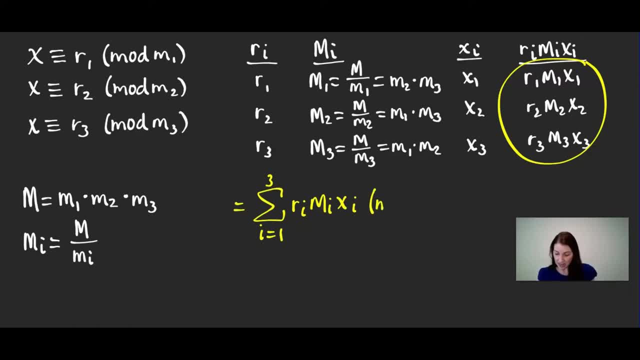 And that sum, when taken in the mod of our unique modulus over here, is going to give us what X is equal to, which is what we're trying to solve for. All right, let's take all of this great information and let's apply it to our original problem. 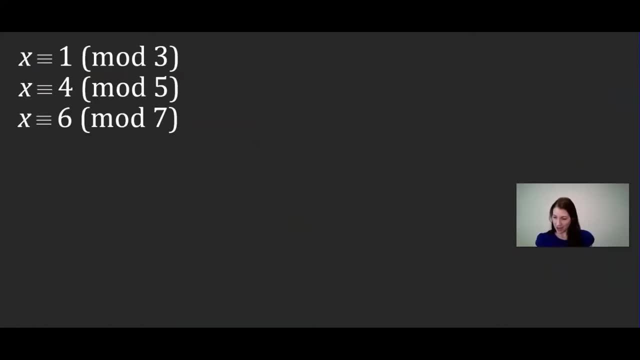 So let's head back and I'll go ahead and move myself back up here and we'll continue on with this problem. So the first thing I write out is I'm going to write out our remainders. So that's going to be 1 and 4 and 6.. 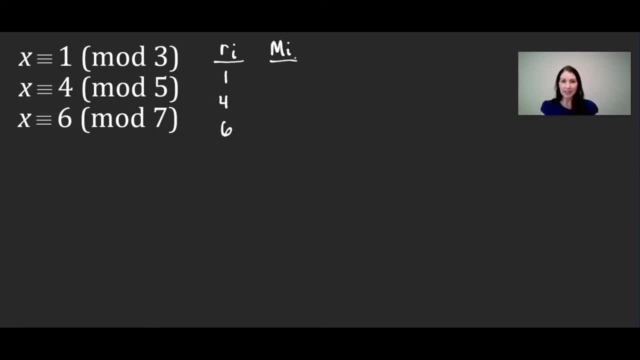 Next are going to be my MIs And MIs, Even though, as you saw, it's really the product of the other two moduli. I am going to write out what that unique modulus M is, because we will need to use it later. 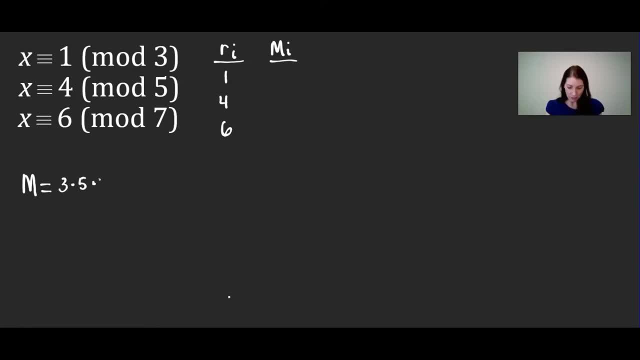 And that's going to be the product of the three moduli, And in our problem here we're going to have 105.. All right, so for our first M1, it's going to be the product of 5 and 7, or 35. 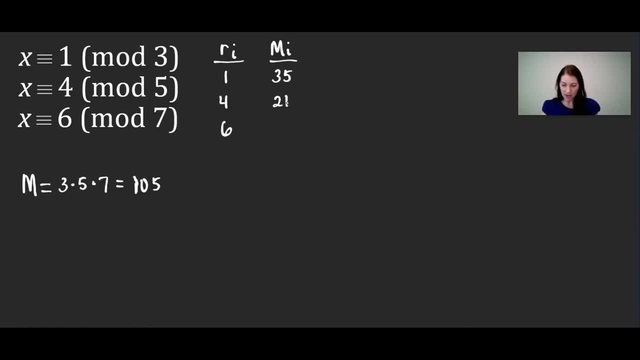 For the next one, it's going to be the product of 3 and 7,, or 21.. And the third one, the product of 3 and 5, which is going to be 15.. All right, now for our inverse. 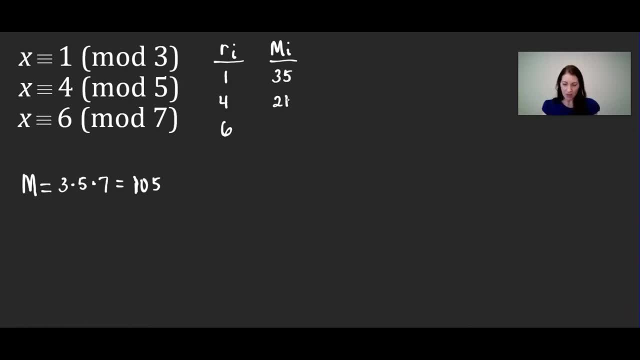 the product of 3 and 7, or 21, and the third one, the product of 3 and 5, which is going to be 15.. All right, now for our inverse, and what we're going to do here is we're going to take the 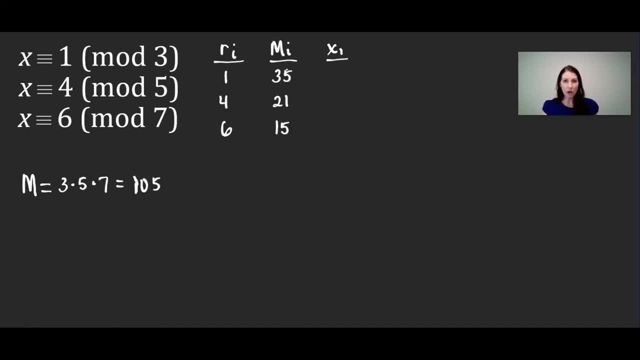 inverse of the m1, m2 and m3.. So for our first one, to find x1, I'm going to take 35, x1 and we know an inverse is that you know, a multiplicative inverse. as we multiply these and with modular arithmetic and a linear congruence, it's going to be the product of 5 and 7 or 35.. So for our next one, 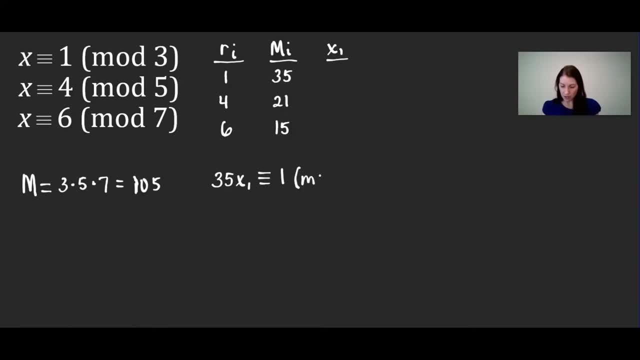 be congruent to 1. and then we want to take mod 3 for this first one and let's see if I solve this. and I know these linear congruences problems can be solved in many different ways, so I'm going to write this in a congruent way. let's see. 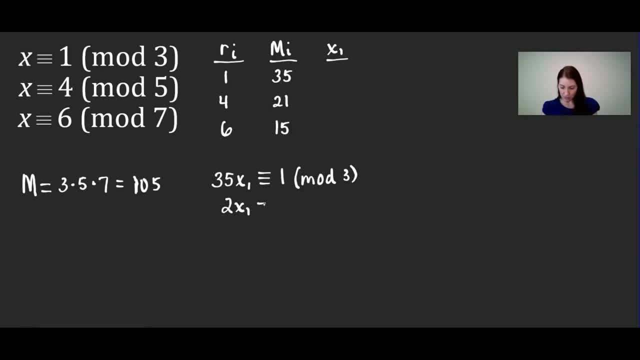 I would have 2. X 1 is congruent to. let's see: add 3, 4, that means X 1. let me go back and include the mod 3 here. that means X 1 is going to be congruent to 2 in mod 3. therefore, 2 is the inverse all. 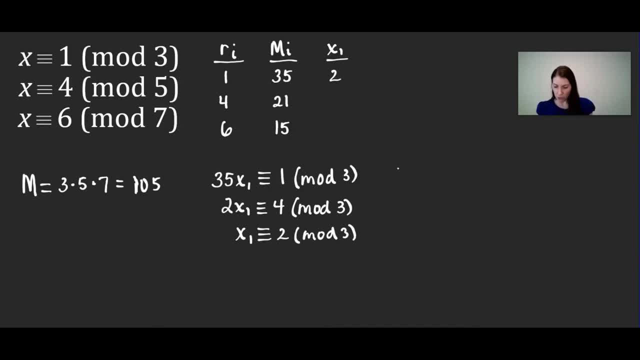 right, let's do the second one. here I would have 21 X 2 because I find in the inverse this would be congruent to 1 in mod m 2, which is 5. let's see if I subtract and somehow it will prevent of Kampfotti Y3 from so. obviously we're going to keep. 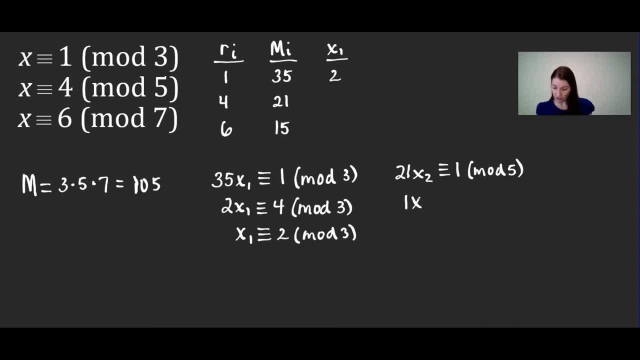 5,. that would give me 1.. X2 is congruent to 1 in mod 5,, so it looks like the inverse is 1.. And then for our last one, 15 X3 would be congruent to 1 in mod 7.. 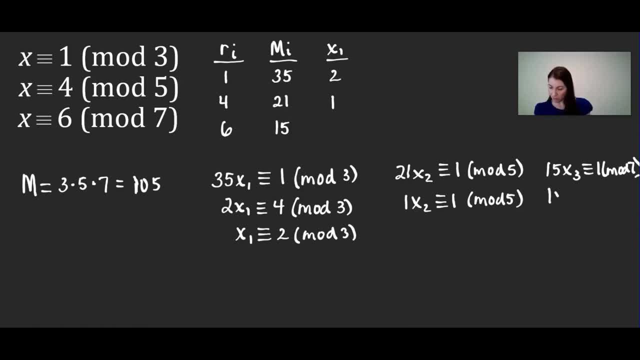 And as I subtract 7, we would have 1. X3 is congruent to 1 in mod 7, so it looks like its multiplicative inverse is also 1.. Now, in that last column, I'm going to take the product of all. 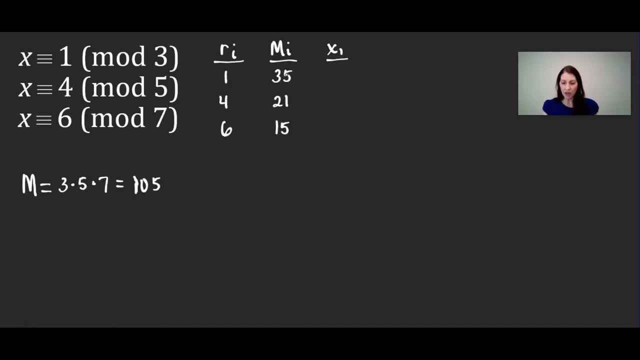 And what we're going to do here is we're going to take the inverse of the M1, M2, and M3. So for our first one to find X1, I'm going to take 35X1.. And we know an inverse is that. 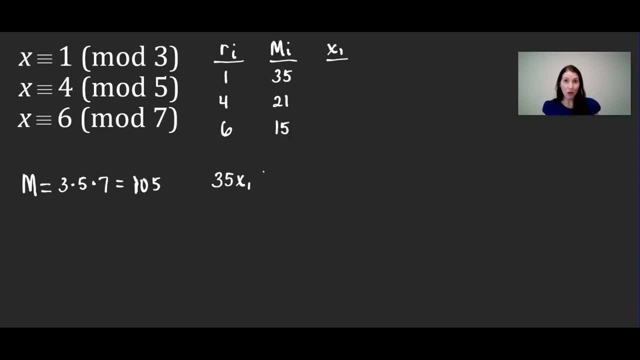 You know, a multiplicative inverse is we multiply these And with modular arithmetic and a linear congruence it's going to be congruent to 1.. And then we want to take mod 3 for this first one And let's see if I solve this. 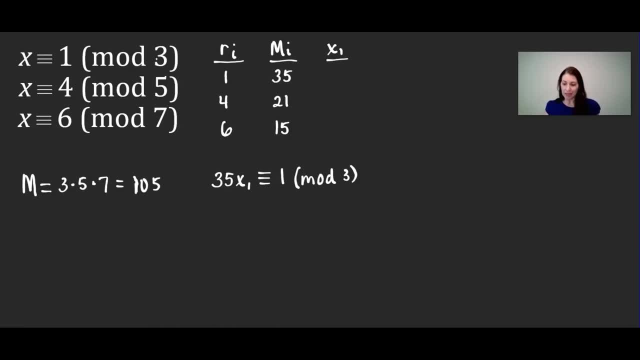 And I know these linear congruences problems can be solved in many different ways, So I'm going to write this in a congruent way. Let's see I would have 2X1 is congruent to. Let's see. 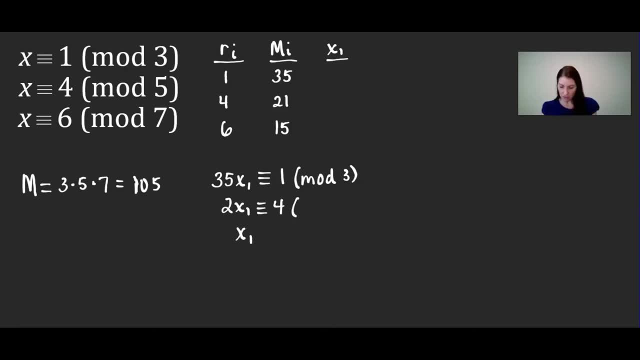 Add 3, 4.. That means X1.. Oh, let me go back and include the mod 3 here. That means X1 is going to be congruent to 2 in mod 3.. Therefore, 2 is the inverse. 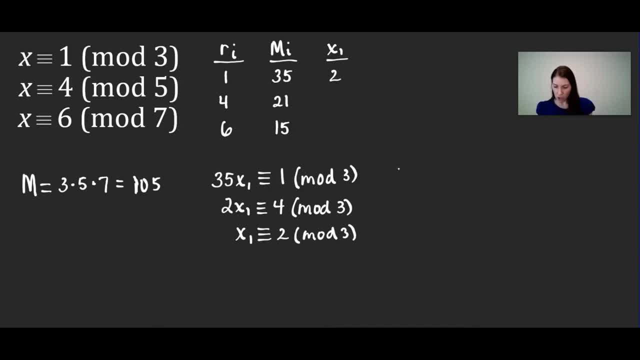 All right, let's do the second one. here I would have 21X2.. And because I'm finding the inverse, this would be congruent to 1 in mod M2., Which is 5.. All right, let's see. 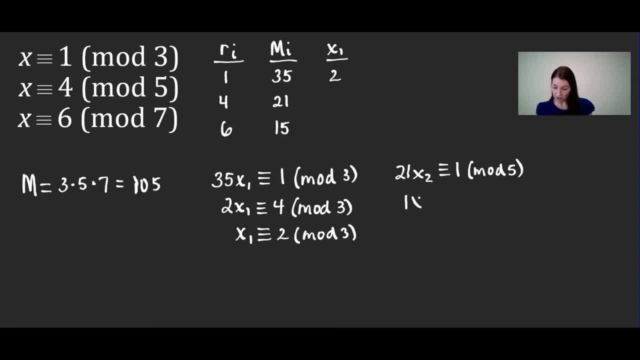 If I subtract 5, that would give me 1.. X2 is congruent to 1 in mod 5.. So it looks like the inverse is 1.. And then, for our last one, 15X3 would be congruent to 1 in mod 7.. 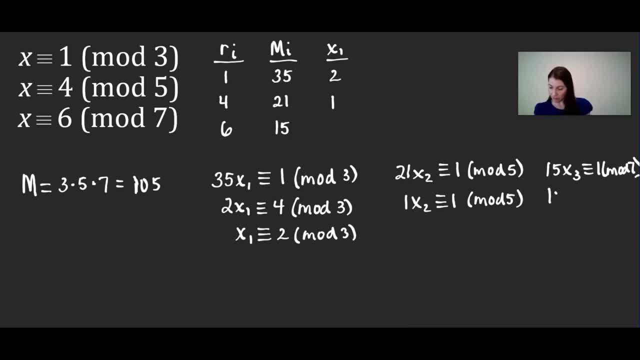 And as I subtract 7, we would have 1X3 is congruent to 1 in mod 7.. So it looks like its multiplicative inverse is also 1.. Now, in that last column I'm going to take the product of all three. 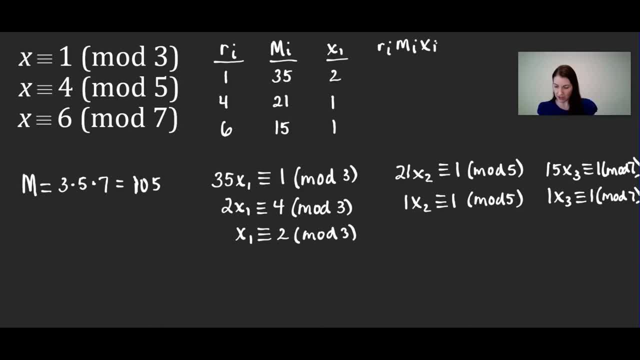 So RI MI, times XI, Let's go ahead and take that product And, by the way, if you think so far the way this is organized and the way that it's laid out, go ahead and give it a like and comment below. 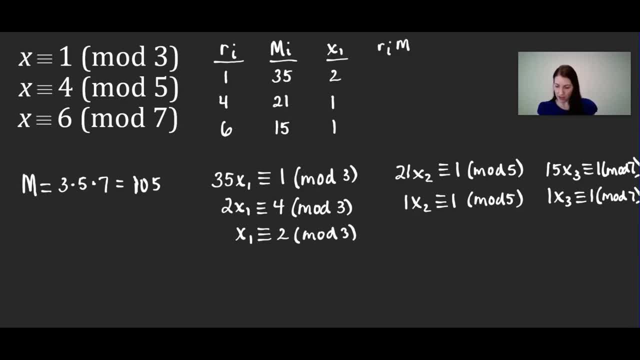 three, So Ri, Mi times Xi. Let's go ahead and take that product And, by the way, if you think so far the way this is organized and the way that it's laid out, go ahead and give it a like and comment below And I'll see you in the next one. Bye. 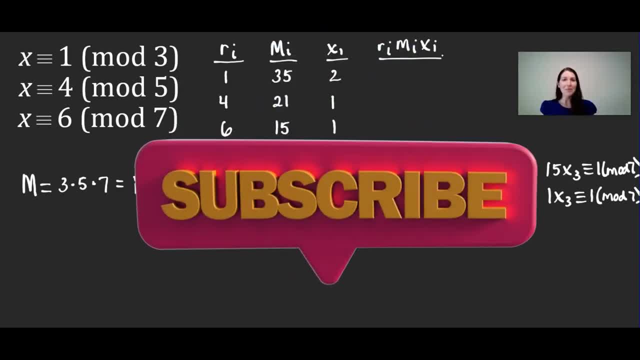 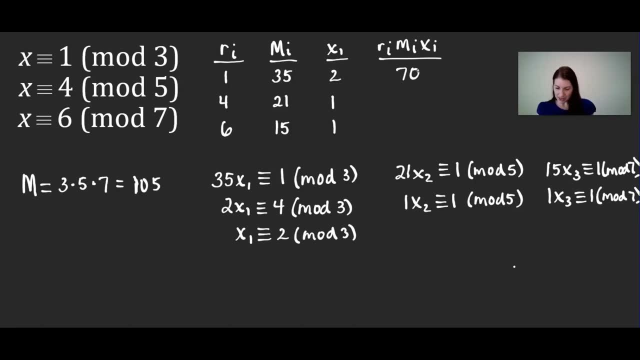 And if you haven't subscribed to the channel yet, make sure to subscribe, because I hope it's explained in a way that is easy to understand. All right now, taking the products, we have 70,, we have 84, and we have 90. And finally, for the grand finale, what we're going to do is we're going. 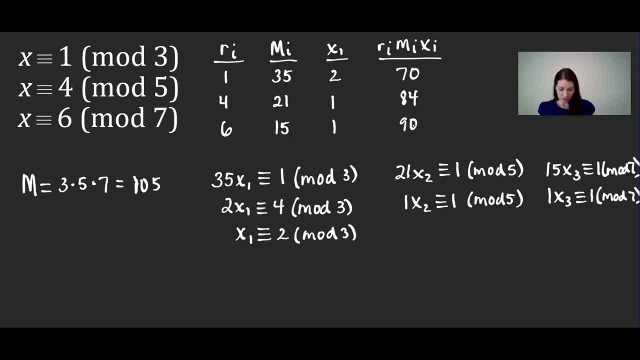 to add up all of those numbers. So if I add up 70 and 84 and 90, this is how I'm going to solve for X. So X is going to be: let's see: if I add these up I get 244.. So to find X, it's going to be 244. 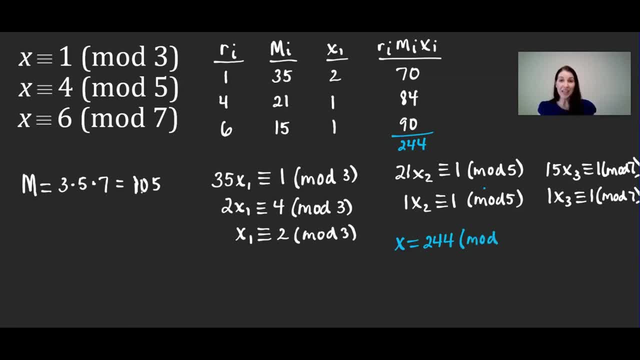 But in my mod of my unique modulus over here, of 105.. So if you find 244 mod 105, you get the final answer of 34 as the value of X. Now I always like to check my answer- I'm big on that- so that I know that if it, you know, seems correct. 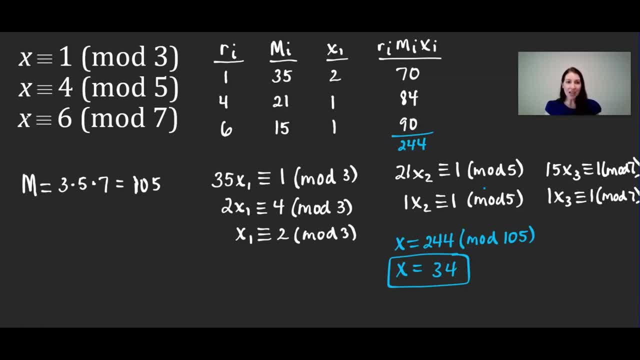 when I plug it in. So I'm going to plug it into the three simultaneous congruences that we started with. So 34 should be congruent to 1 in mod 3. So the remainder should be 1 and 33.. Yep: remainder 1.. 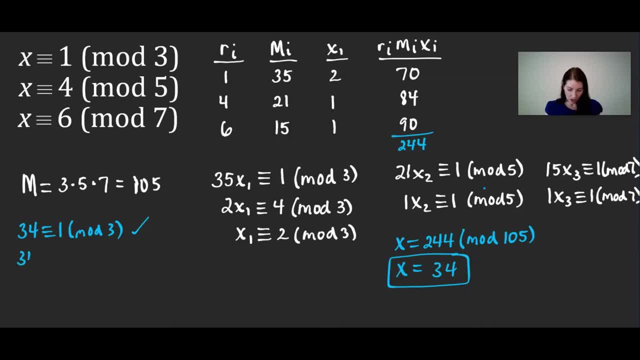 Great, that one works. Okay, 34 should be congruent to 4 in mod 3.. Mod 5. And let's see, goes in, gets 30 with 4 left over. Yep, that one works, And then 34 should be. 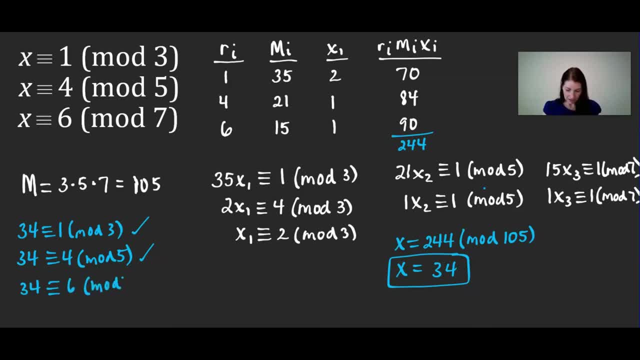 congruent to 6 in mod 7.. And once again, yep, that would be 28 with a remainder of 6.. So it also works there. So, as you can see, we did the check, 34 looks like it works And I think this is going to work. 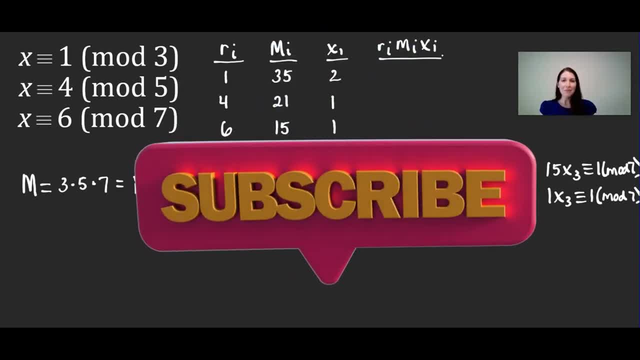 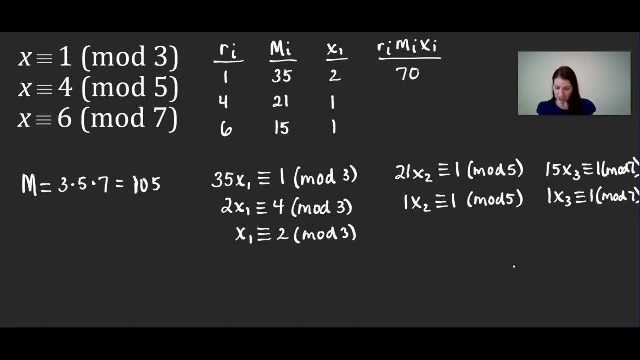 And if you haven't subscribed to the channel yet, make sure to subscribe, Because I hope it's explained in a way that is easy to understand. All right now, taking the products, we have 70.. We have 84. And we have 90.. 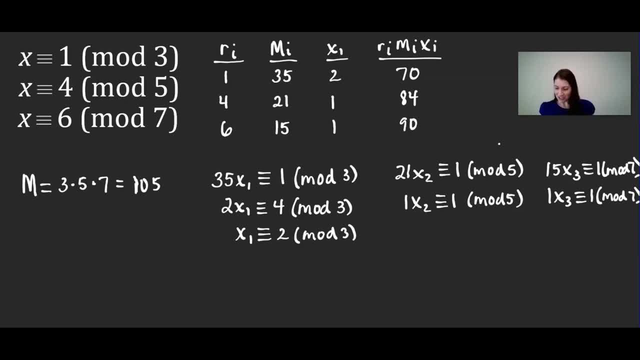 And finally, for the grand finale, What we're going to do is we're going to add up all of those numbers. So if I add up 70 and 84 and 90,, this is how I'm going to solve for X. 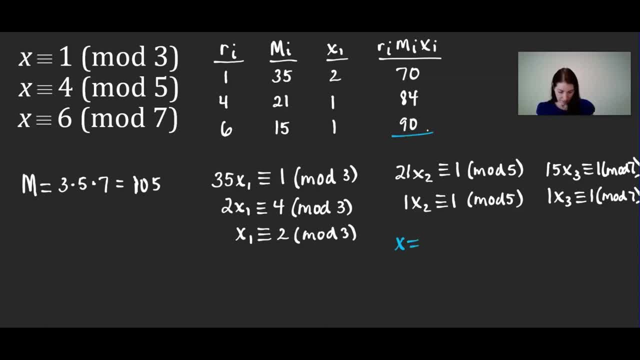 So X is going to be. Let's see. if I add these up I get 244.. So to find X, it's going to be 244. But in my mod of my unique modulus over here, of 105. So if you find 244 mod 105, you get the final answer of 34 as the value of X. 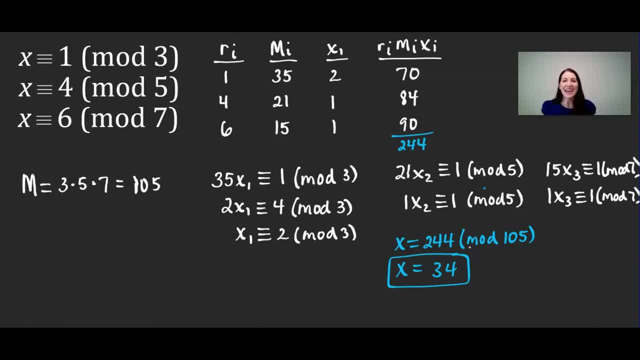 Now I always like to check my answer- I'm big on that- So that I I know that if it, you know, seems correct when I plug it in. So I'm going to plug it in to the three simultaneous congruences that we started with. 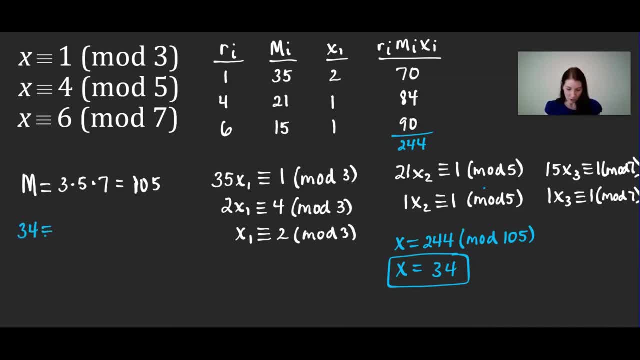 So 34 should be congruent to 1 in mod 3.. So the remainder should be 1 and 33.. Yep, remainder 1.. Great That one works Okay. 34 should be congruent to 4 in mod 5.. 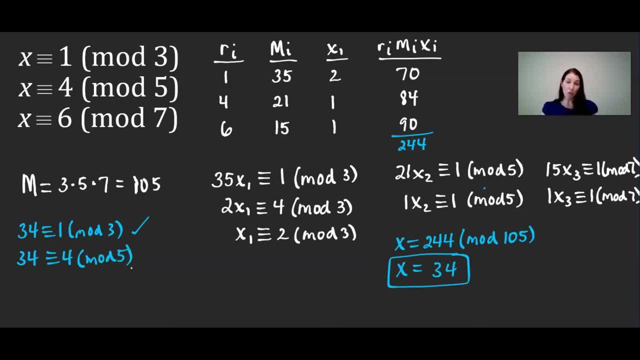 And let's. Let's see: Goes in gets 30 with 4 left over. Yep, that one works. And then 34 should be congruent to 6 in mod 7.. And once again, Yep, that would be 28 with a remainder of 6.. 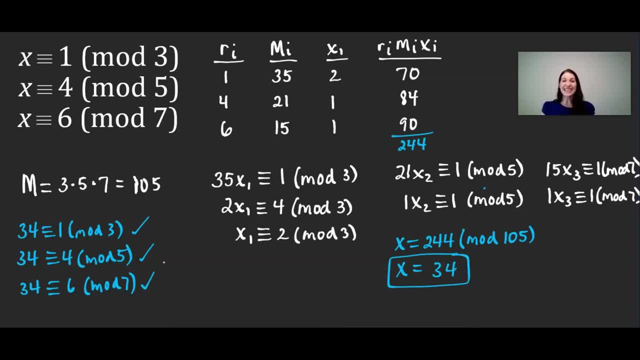 So it also works there. So, as you can see, we did the check. 34 looks like it works And I think this is just like a nice organized way to use to use Sun-Zoo's Theorem. I hope you found this video useful. 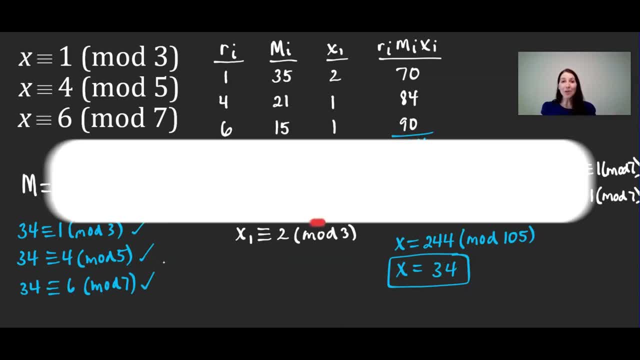 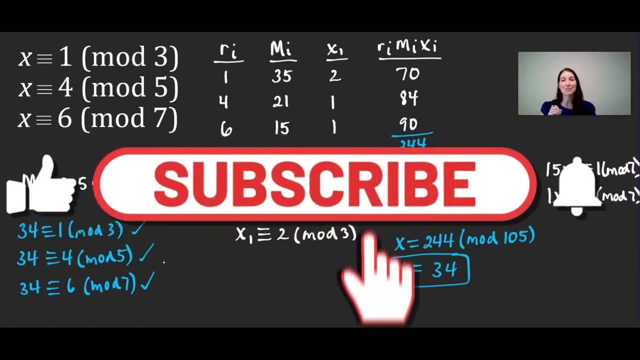 Again, if you did, make sure to give it a thumbs up Comment below about any questions you have or just any comments that you'd like to give. And again, if you haven't subscribed, make sure to subscribe in the lower right-hand corner. 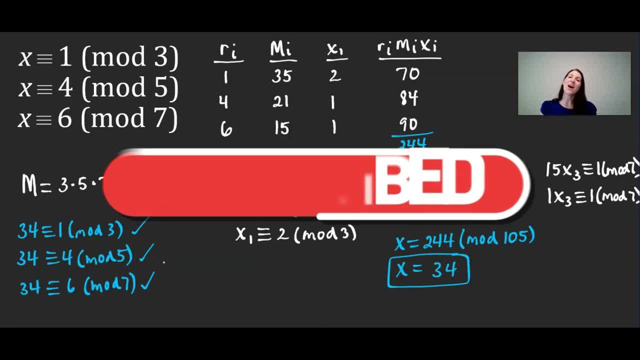 so that you can see weekly math videos. I hope you all have a wonderful day. See you in the next video.